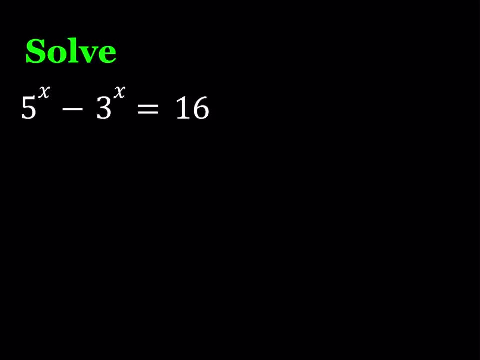 great. So since 5 is a higher base, I'm going to divide everything by 5 to the power x. So we're going to start by dividing everything by 5 to the power x. It'll become clear why I'm doing this In a little bit. let's divide 5 to the power x by 5 to the power x, and then 3 to the. 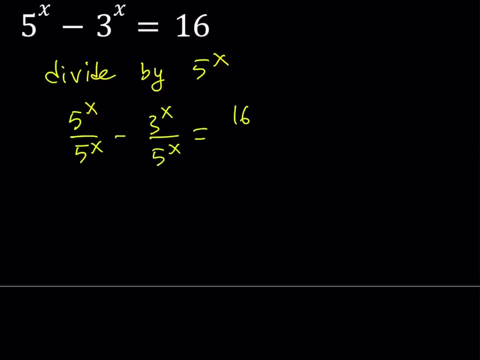 power x by 5 to the power x. So we're going to divide everything by 5 to the power x and then 16 by 5 to the power x. Obviously, 5 to the power x is never 0, unless x is negative infinity or. 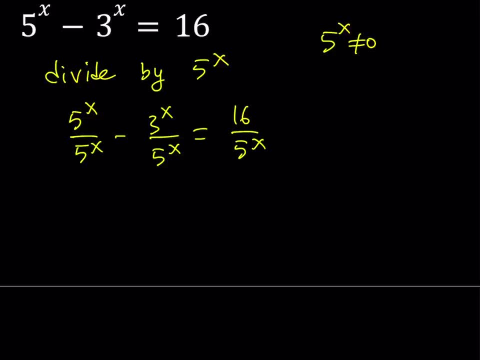 approaches negative infinity or whatever. It can never be 0. It's always positive. So this is okay to do Now. 5 to the power x divided by 5 to the power x is obviously 1, as you know. And this: 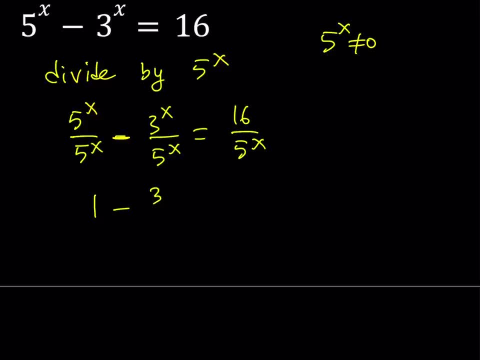 expression, because they have the same exponent, can be written as 3 to the. I mean 3 over 5 to the power x, And the right-hand side of the equation is going to be 3 over 5 to the power x. 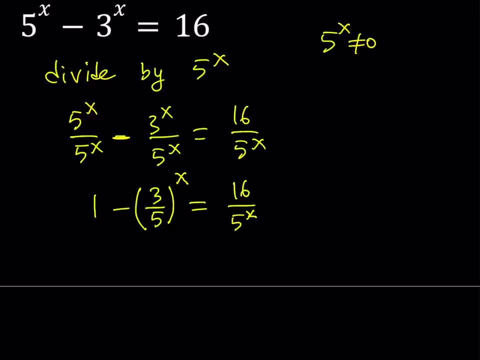 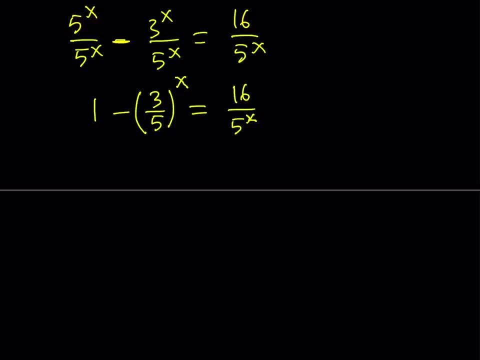 The left-hand side is what it is: 16 divided by some power of 5.. Okay, now, when you look at this equation carefully, this equation has an interesting feature, or property, or whatever you want to call that. What is it? It is the fact that 3 over 5 is less than 1.. Okay, so what about it? right? 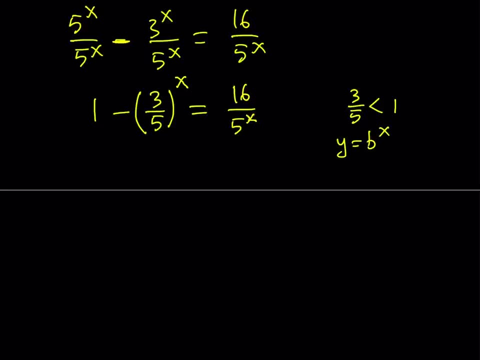 If you have an exponential function- y equals b to the power x and b is less than 1, then you're basically talking about a decreasing function, as you know from the previous video. So you're going to have some exponential equations If b is greater than 1, or I should say between 0 and 1,. 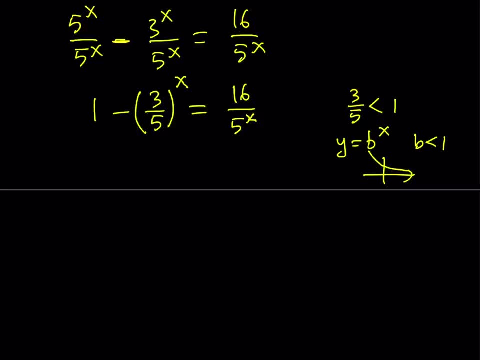 wait a minute, okay. If b is greater than 1, sorry about that. obviously we want b to be positive, so b is positive in this case. So if b is between 0 and 1, then our function is decreasing, If b is. 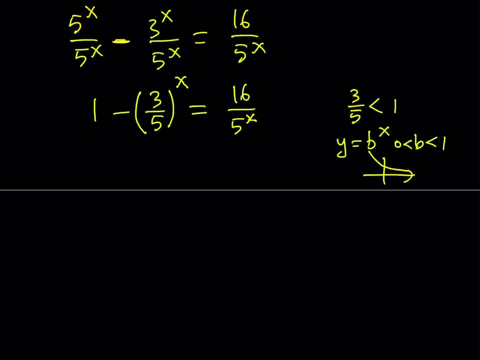 greater than 1, then it's going to be increasing, as you know, from e to the power x, or 2 to the power x or whatever. In this case we have a decreasing function, Great. So, 3 over 5 to the. 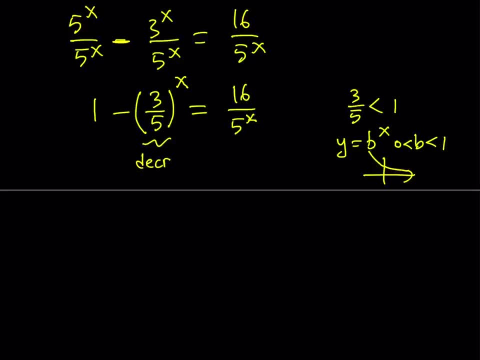 power x is decreasing. This is decreasing, So if b is greater than 1, then it's going to be increasing. Let's call that d, e, c, r, And on the right-hand side I have 16 divided by 5, to the power x As. 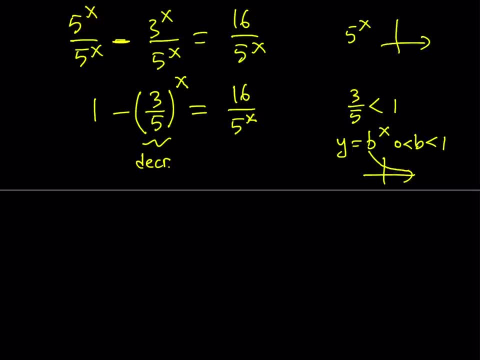 you know, 5 to the power. x is increasing. Why? Because 5 is greater than 1, so you're going to get something like this: So the denominator of a function is going to increase without any bounds. So 16 divided by that is going to decrease. This is also a decreasing function. 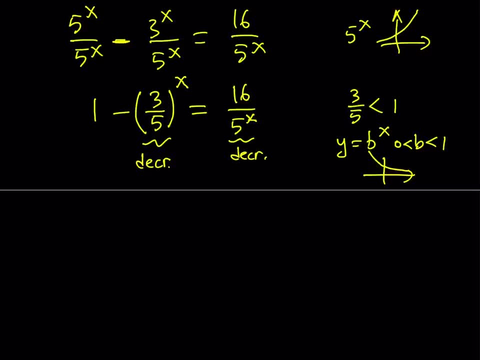 So what is the big deal about it? Like you have two decreasing functions- No, The left-hand side- we are subtracting the decreasing function from 1.. In other words, we are negating the function. Notice the negative sign: If you multiply a decreasing function by negative 1, it is going. 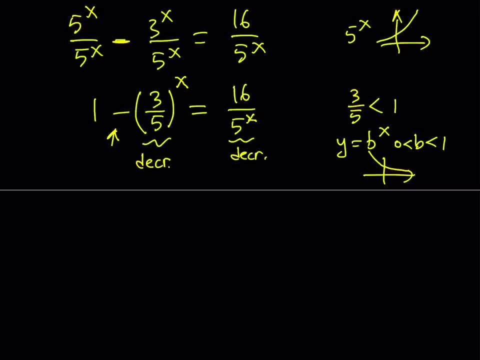 to be increasing because you're basically flipping it right. So we have an increasing function plus 1.. Plus 1 is not going to make any difference, It's just going to move it up. So we have an increasing function on the left-hand side and a decreasing function on the right-hand side. What? 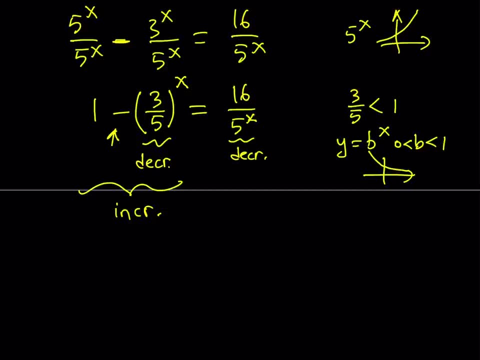 is that supposed to mean? Well, these functions are only going to intersect at one point, if they do intersect. So we have an increasing function on the left-hand side and a decreasing function on the right-hand side. So we have an increasing function on the right-hand side. So we have an 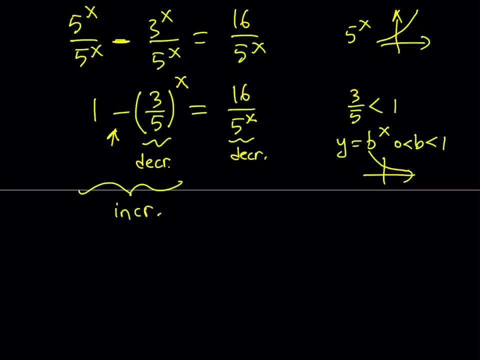 increasing function on the left-hand side and a decreasing function on the right-hand side intersect at all. right, Great. So that's one way to look at the problem. I want to show you an alternative approach here, Not a whole different method. but if you add 3 over 5 to the power x to 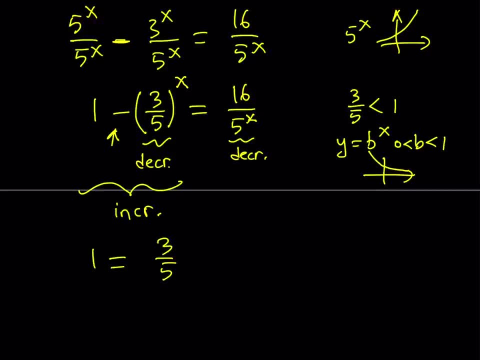 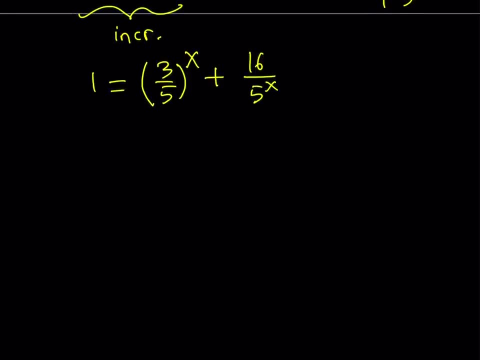 both sides. you're going to get the following: 3 over 5 to the power x, plus 16 over 5 to the power x. Now look at it from this perspective. On the right-hand side, we have two decreasing functions. 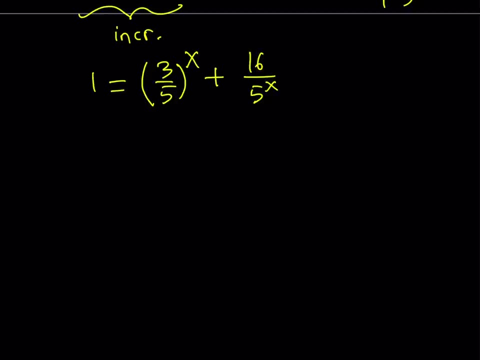 If you add two decreasing functions then you get a decreasing function. Why? Because their first derivatives are negative and the derivative of the sum is the sum of the derivatives and they're going to be negative. So when you add two negative numbers, 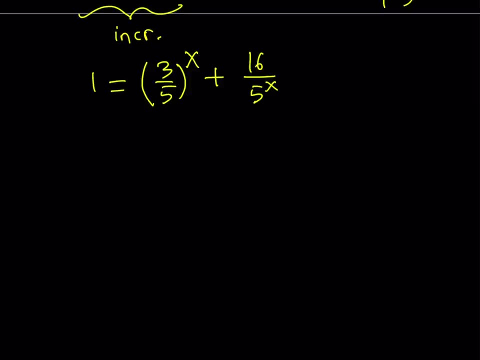 you're going to get a negative number, Or there is another way to prove it as well, but I just used calculus because it's easier. So we have a decreasing function, we have another decreasing function and the sum is also decreasing. So on the right-hand side I have a function that is: 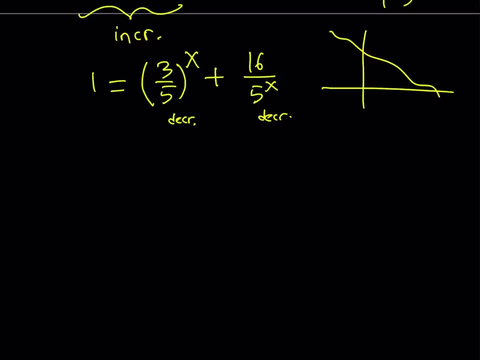 decreasing, no matter how it goes. And on the left-hand side I have a constant function, So that means this function is going to be a horizontal line. So you have like a decreasing function and a horizontal line. Now let's go ahead and make it a little bit more accurate. Sorry, I don't have a Desmos drawing of. 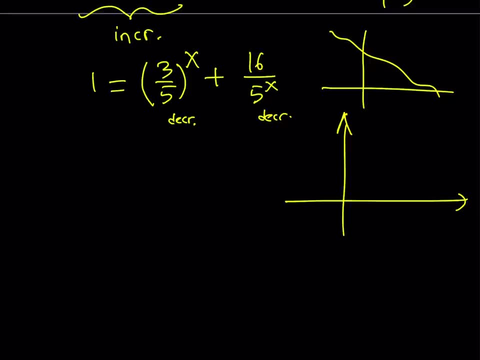 this, but I'm just going to do a hand drawing. I hope you don't mind. If you just evaluate our function as at: x equals 0, for example, this is going to be 1 plus 16.. So our y-intercept is going: 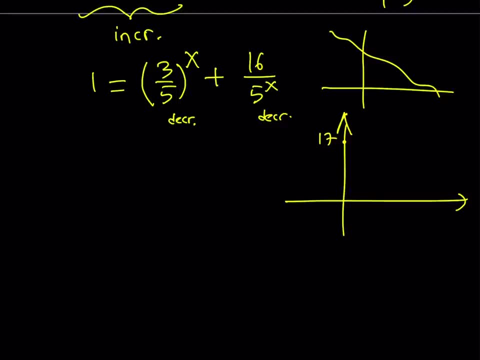 to be at 70.. Pretty high, right, And are we going to have an x-intercept? Who knows Now what happens if x approaches infinity? right, As x approaches infinity, this is going to approach 0, and this is. 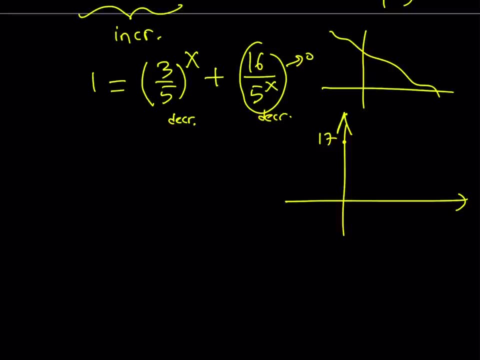 going to approach 0.. So our function is going to approach 0, but since everything is going to stay positive, our function is kind of going to stay above the x-axis, So something like that Doesn't really matter. The details are not that important. But we do have another function which is: 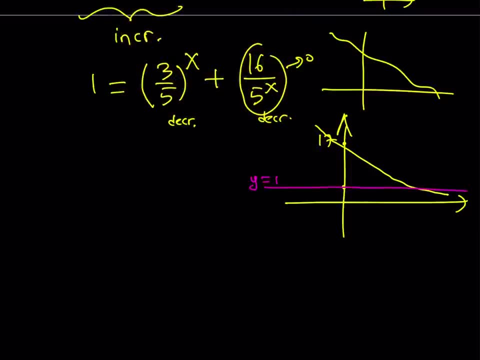 horizontal right, And that is y equals 1.. This is y equals 1.. This is y equals 3 over 5 to the power of x, plus 16 over 5 to the power of x. So we have a decreasing function and we have a 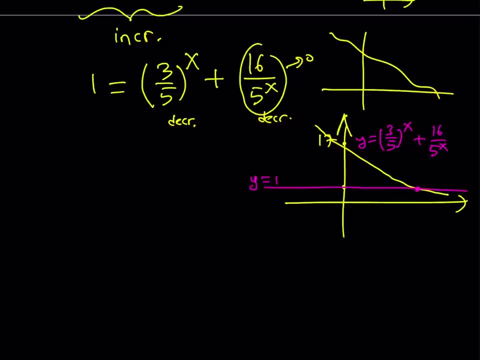 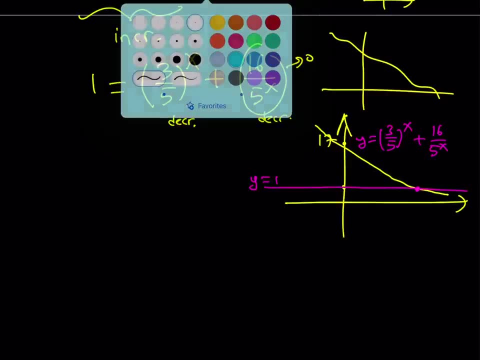 and they will intersect at one point only. That's the whole point. okay, All right, great. So now what is that supposed to mean? It means that there's only one solution to this equation. So let's go ahead and write our original equation one more time. Our original problem was 5 to the 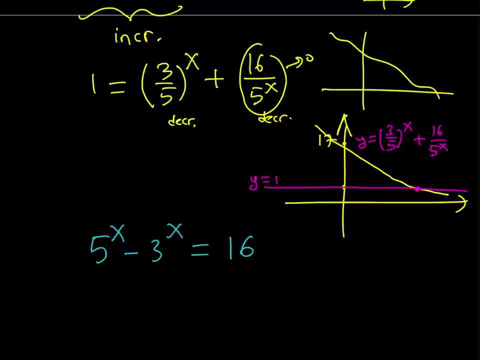 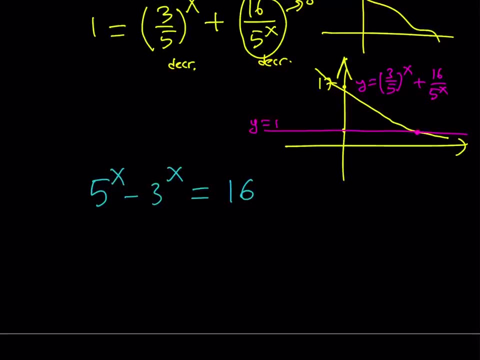 power of x minus 3 to the power of x equals 16.. So we're basically saying that this equation has a single solution. And how do you find that? Guess and check Is guess and check a problem solving method. Yes, it is Okay. 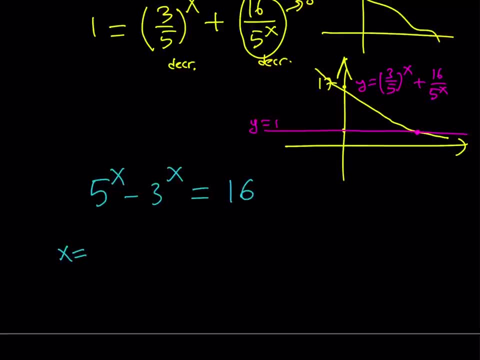 You may disagree if you want, but that is a problem solving method. So if x is equal to, for example, 1, I get 5 minus 3.. That's too small. How about x equals 2?? Let's see 5 squared minus. 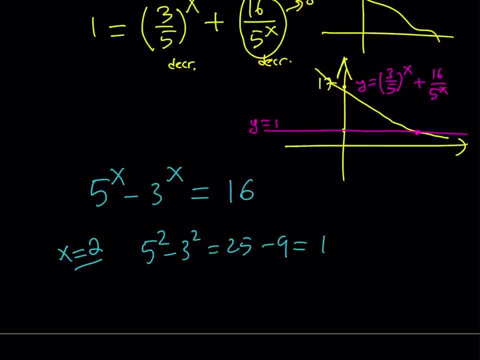 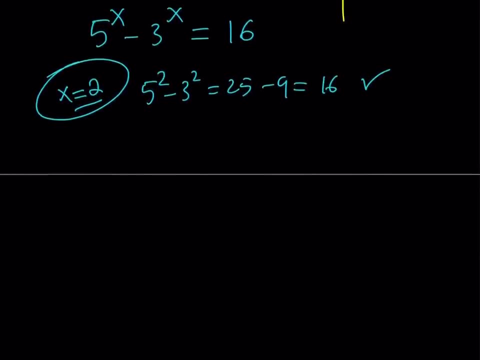 3 squared is 25 minus 9, and that is equal to 16.. Bingo, We got it, Okay, great. So x equals 2 is a solution, and x equals 2 is the only solution to this equation. And this brings us to the end. 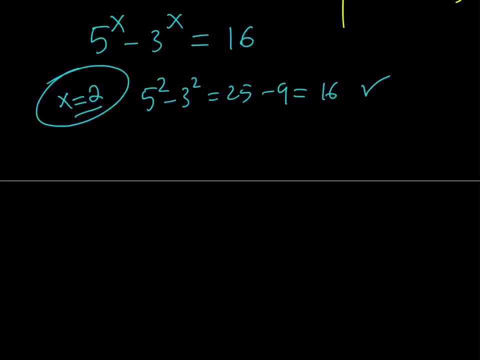 of this video. I hope you enjoyed it. Please let me know. Don't forget to comment, like and subscribe. I'll see you tomorrow with another video. Until then, be safe, take care and bye-bye.